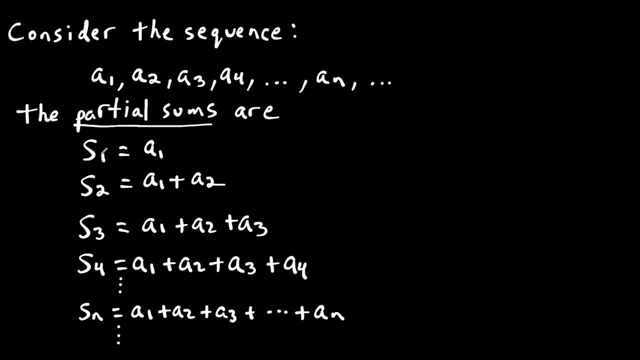 could just go on forever. But the partial sums. what we have here is the first partial sum is just the first term of the sequence, but the second partial sum we add the first two terms of the sequence and then for the third one we add the first three terms and by the time we get to the 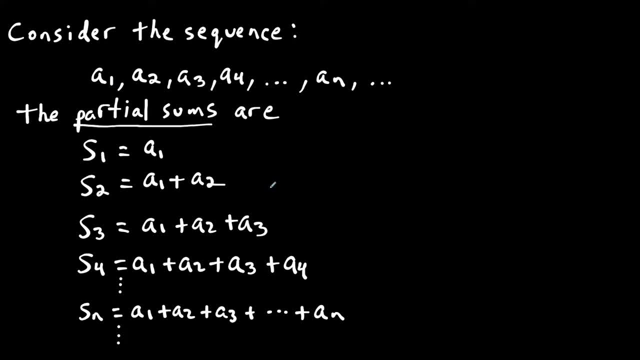 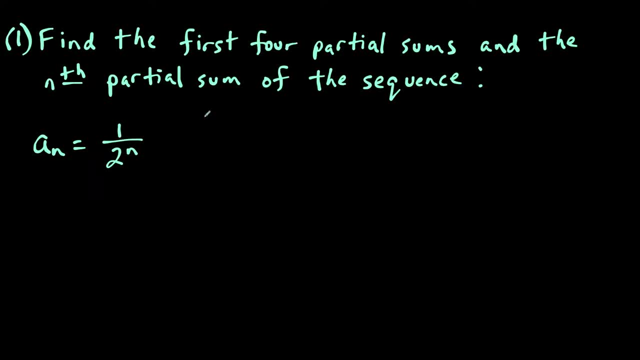 nth partial sum, we're adding the first n terms of the sequence. So that's the general idea, but let's look at a few examples. So, for all the questions that I'll go over, we're going to find the first four partial sums and the nth partial sum of the given sequence. So what I like to do for questions. 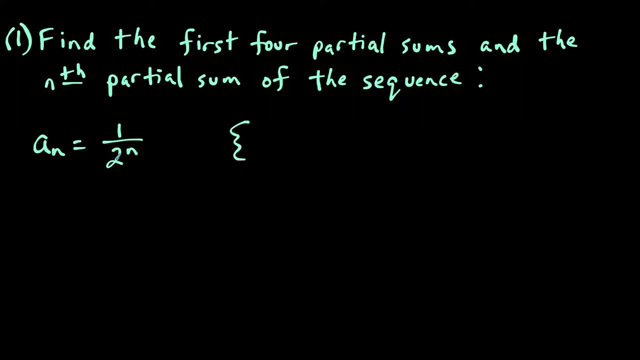 like this is. I like to expand the sequence and see that if I were to plug in 1, I would have 1 over 2 to the first power, which would just give us one half. but if I plug in n equals 2, I would have 1. 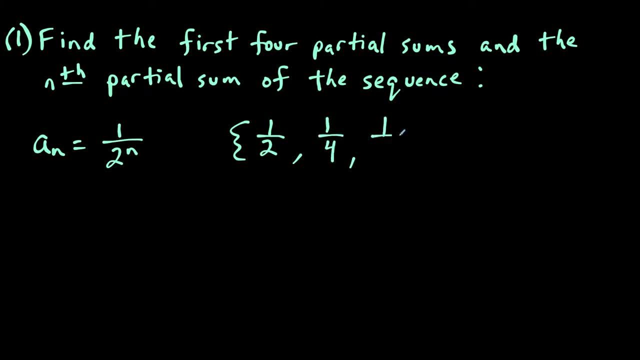 over 2 squared, which would give us 1 over 4. and then this would be: next would be 1 over 8, when I do 1 over 2 to the third, 1 over 16. And then this would continue on and on. so this is kind of like the expansion of our sequence. so now, 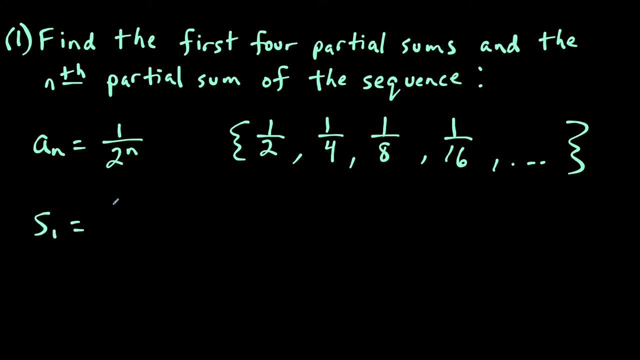 when I want to find the first partial sum, that's just the first term of the sequence, which is one half, but the second partial sum I would do one half plus one fourth, and I'm just going to make common denominators here. if I do times 2, times 2, I'm going to have 2 over 4 plus 1 over 4, which. 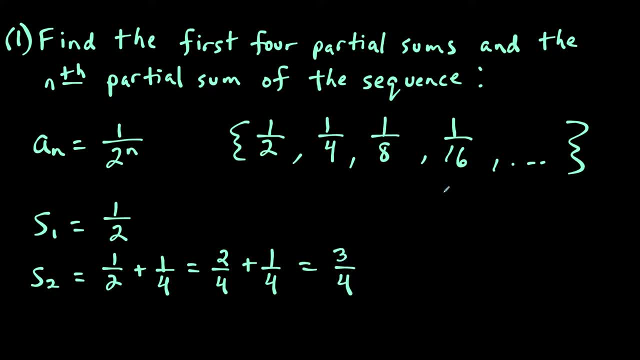 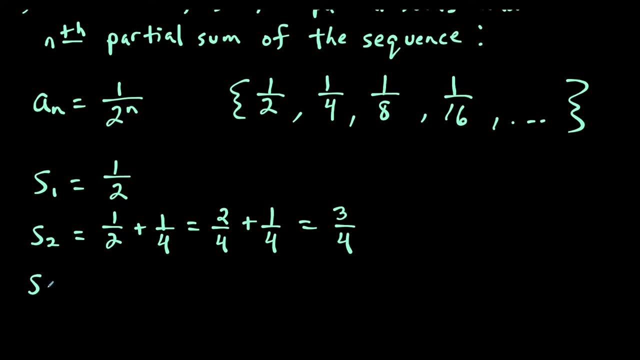 is equal to 3 over 4.. That's why it's a good idea to find four partial sums. you could usually spot it by, like the third, but sometimes it helps to go out another one. so now I'm going to add the first three terms. so we'd have: 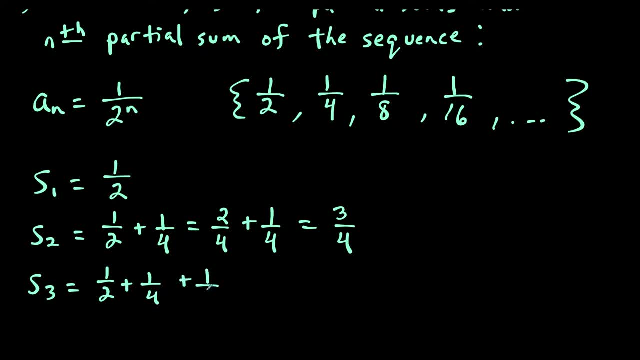 one half plus one fourth plus one eighth and if we work this out, we find common denominators. that would be 4 over 8. for the first fraction, 1 over 4. we could write as 2 over 8, and 1 over 8 will keep. 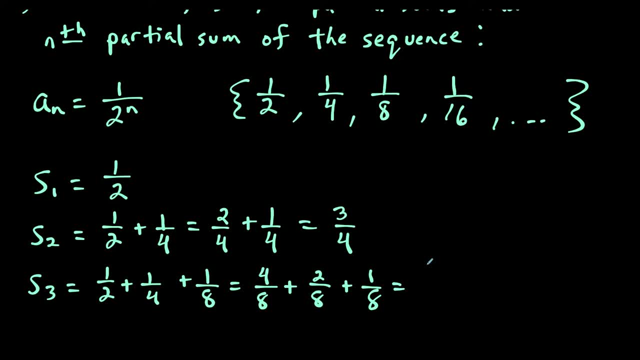 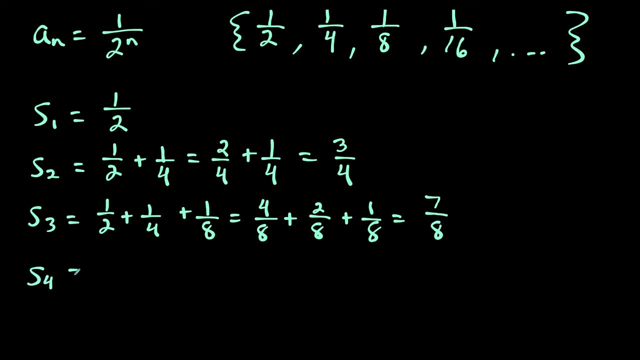 the same. so they have all matching denominators and that would give us 7 over 8.. So by now you have the pattern and notice here that for the fourth partial sum I could probably just go forward with this. so what I notice here is that it's 2 to the power, 3 on bottom, and then I just subtract one. 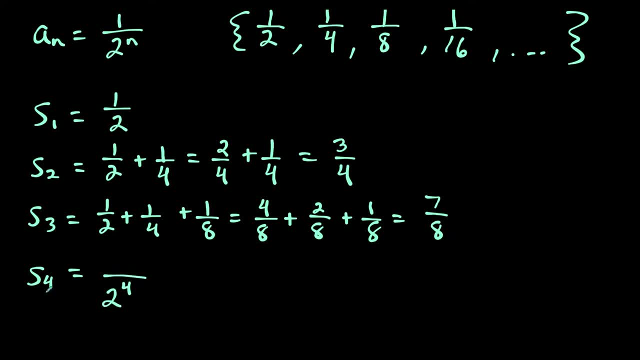 for the thing on top. so here I would have 2 to the fourth power, because that's the subscript. here we have the subscript. 4 would give me 2 to the fourth power, and then on top I'm going to have one less than that. so I'd have 2 to the fourth minus 1. so in the denominator I'm going to have 16, and if I 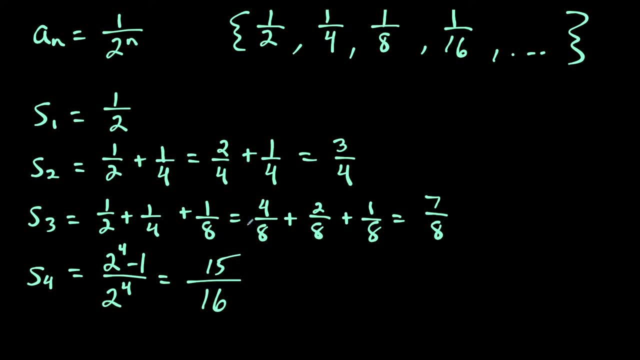 do one less than 16, that's 15, okay. so once again, like usually, by the third term it's a little bit obvious what the pattern is. so now we want to find the nth term, so we want to generalize it for any partial sum. so what we're going to do is we notice here once again that what we have is the subscript. 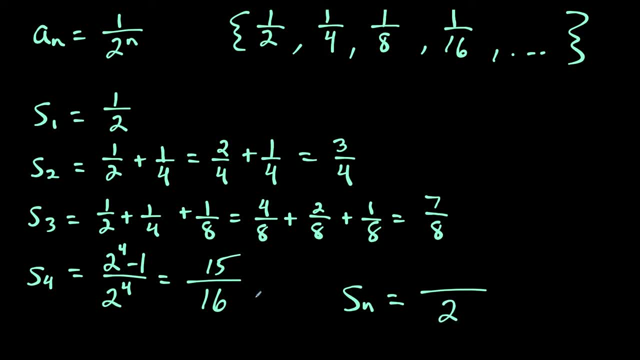 tells you the power of 2 in the denominator. so I'd have 2 to the power n and then the numerator is 2 to the power n, so I would make this 2 to the n minus 1 like this. so this would be our nth partial. 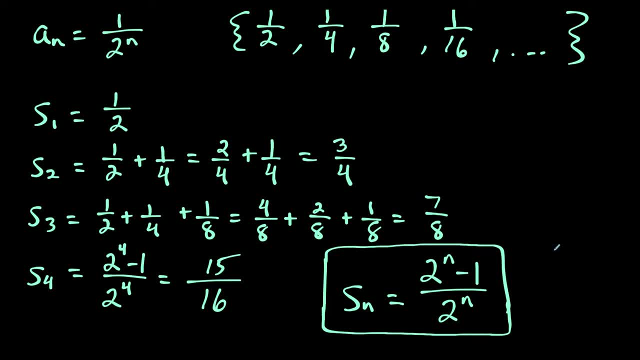 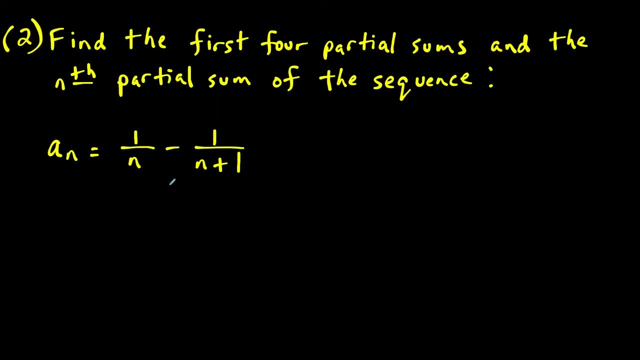 sum. so one of the major skills that you need for this topic is you have to be able to spot the pattern. so let's look at another example. except this time around, this is going to be our sequence: 1 over n minus 1 over n plus 1. so what we'll do is we'll find the first partial sum by just looking. 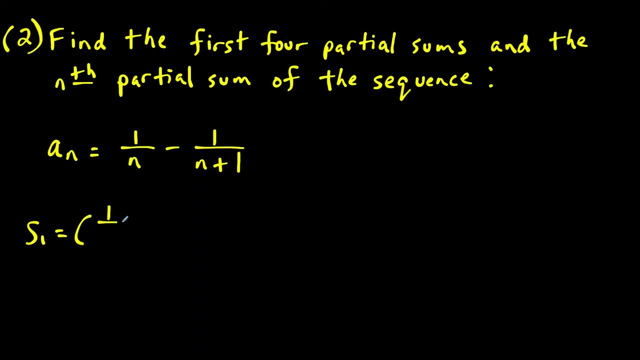 at the first term at n equals 1, so this would give us we would have 1 over 1 minus 1 over 1 plus 1 is 2. so this is our first partial sum and we could simplify this here. but you're gonna see in a. 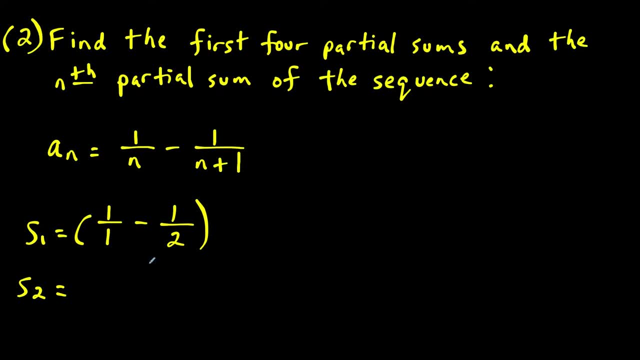 moment that sometimes it's better to simplify after you plug in instead of plug in and then simplify it. so, as sub 2 would be the result of me taking the sum of the first two terms, so that means I would plug in n equals 1, which would give us 1 over 1. we could just call 1 so we have 1. 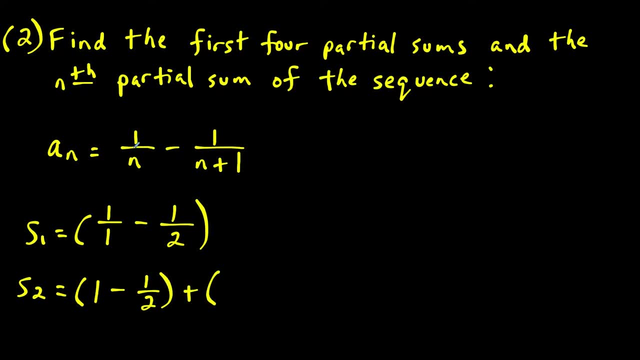 minus 1, half plus. but now if we plug in, n equals 2, 1 over 2. minus 1 over 2 plus 1 is going to give us 1 over 3, and one thing to notice here is that minus a half and plus a half cancel out, and this is going to. 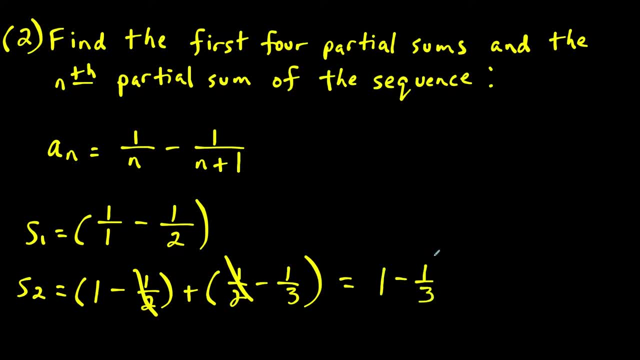 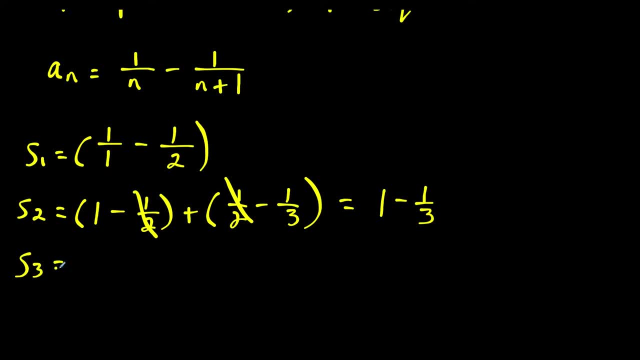 equal 1 minus 1 third. now what we could do from this step is: you might start to notice what's going on here, but just to be safe, we'll check one more. so we would have 1 minus 1 half plus one half minus a third. so those are the first two terms, but now we would just plug in n equals 3 and. 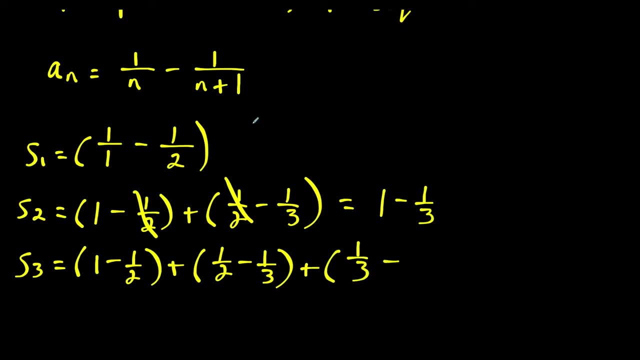 that would give us over 3 minus 1. over 3 plus 1 is 1 over 4.. So by now it might be obvious what the pattern is, because minus a half plus a half cancels. but now minus one third plus a third cancels, and we would 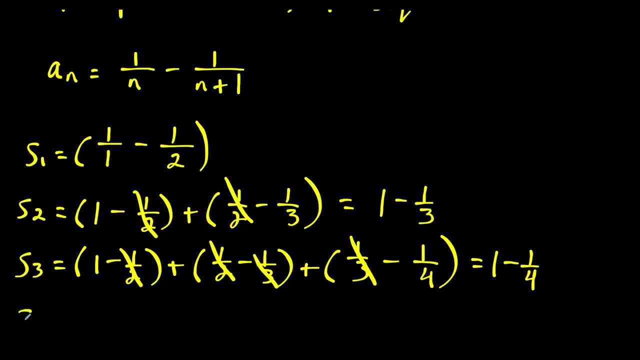 be left with 1 minus a fourth. So, without thinking too much, I think I could see what the pattern is here. We're going to start with 1 and we're going to have minus 1 over and now look for the relationship between the subscript of the partial sum. So we have a subscript of 3 and we wind up. 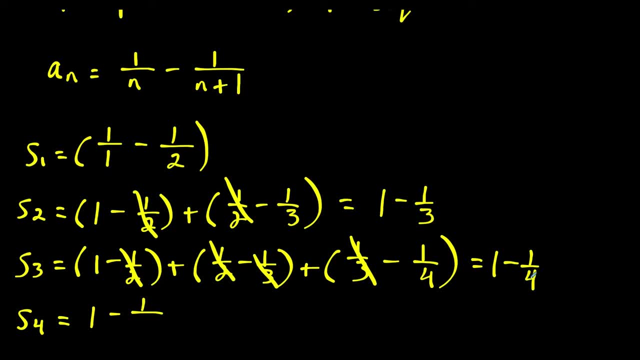 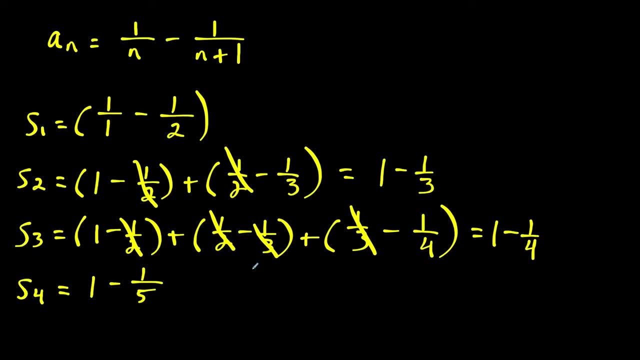 with a denominator of 4.. So it looks like the trailing denominator is going to be 1 more than the subscript. So this time around we'd have 1 minus 1 over 5.. So then, when we want to find the nth partial sum, so just give ourselves a little space here. when we want to find the nth partial, 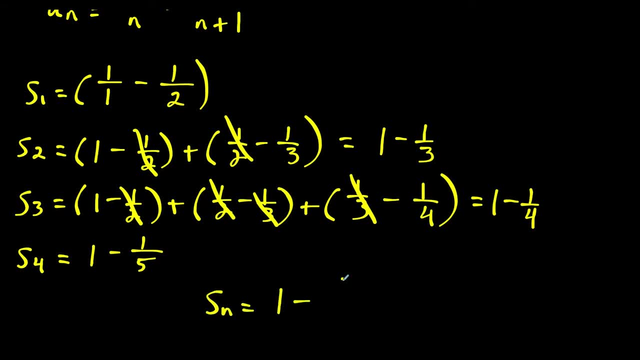 sum. what we could do is we have 1 minus 1 over and once again the trailing denominator is 1 more than the subscript. So we have 3 giving us a trailing denominator of 4, 4 gives us a trailing denominator of 5.. 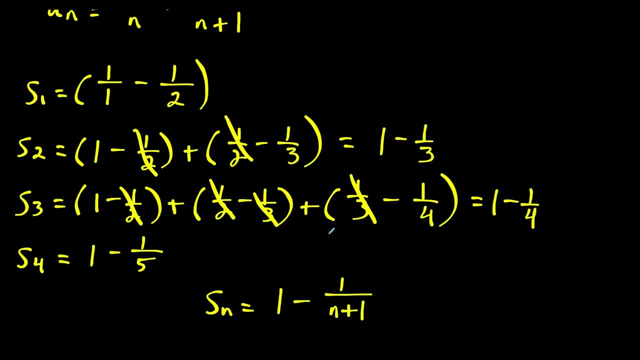 So n would give us a trailing denominator of n plus 1.. So we could leave our answer like this. or if we actually simplify this, 1 minus a half is a half. 1 minus one third is two thirds. 1 minus one fourth would give us three fourths, and if I did 1 minus a fifth, that would give us: 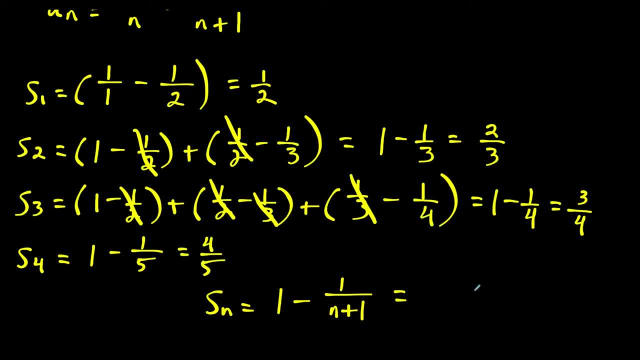 four, fifths. So we could also see here. another way of expressing this is that the subscript goes in the numerator, So that would be n over. the denominator is 1 more than that. Okay, so this could be expressed as 1 minus 1 over n plus 1.. 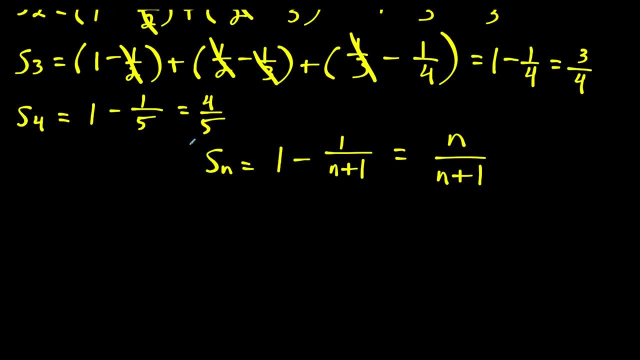 Or we could express it as n over n plus 1.. Now, just know, if we wanted to verify this here, just to be sure, is we could do the actual algebra and show 1 minus 1 over n plus 1 is equal to n plus 1 over n, plus 1 minus 1 over n plus 1.. And if we work this out, we have 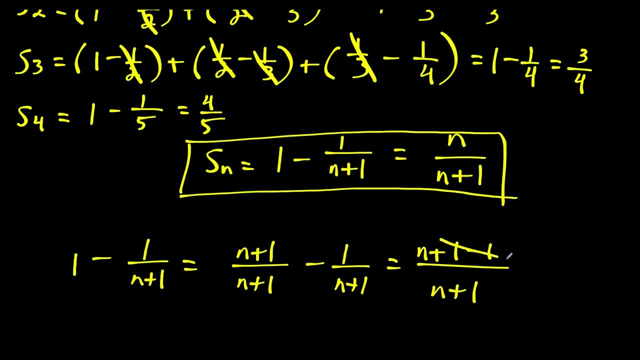 n plus 1 minus 1 over n plus 1.. 1 minus 1 cancels and it still gives us n over n plus 1.. So I'm confident that this is our formula for the nth partial sum. So for the third. 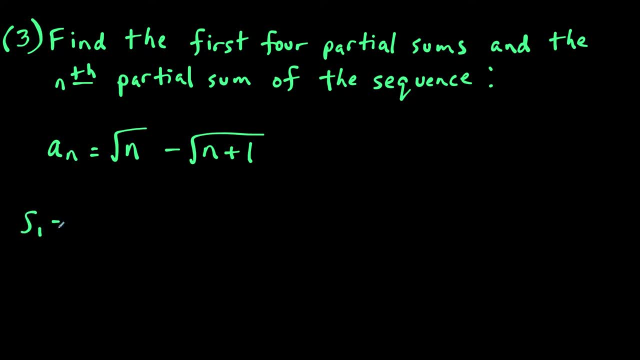 example here We could make a list of the sequence or we could just plug this in as we go: The first partial sum is just the first term of the sequence. So we would have square root 1 minus square root of 1 plus 1 gives us 2.. So this would just give us 1 minus the square root. 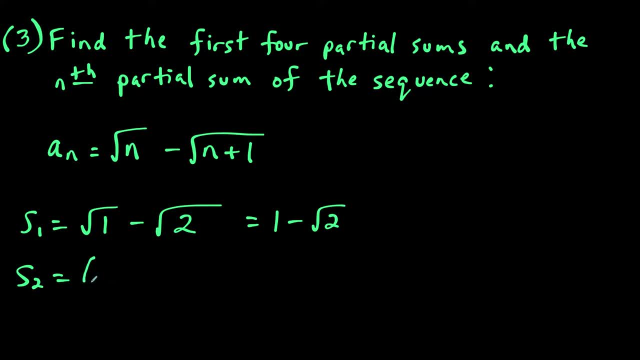 of 2.. The second partial sum: we would take 1 minus the square root of 2 and add the result of plugging in n equals 2, which would give us square root of 2 minus the square root of 2 plus 1 is square root of 3.. And it's the same pattern as before: Minus root 2 plus. 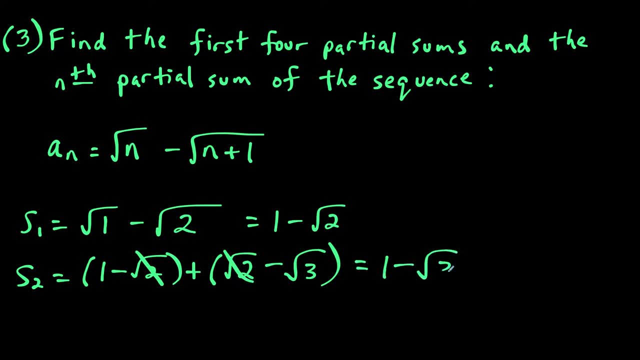 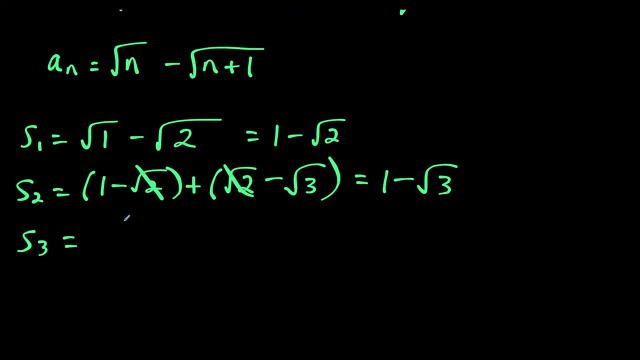 root 2 cancels, giving us 1 minus radical 3.. So now we'll find the first 4 partial sums and then we'll use that to find the nth one. So if we go for the third partial sum, we're going to have 1 minus root 2 plus root 2 minus root 3.. And then plus we plug in n equals. 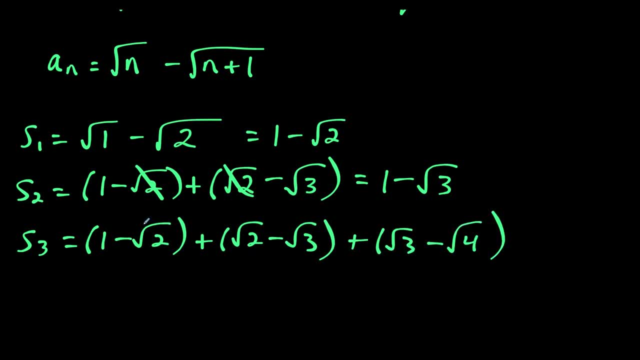 3 and we're going to have root 3 minus root 4.. So here, minus root 2 plus root 2 cancels. minus root 3 plus root 3 will cancel and we'll be left with 1 minus square root of 4.. Now 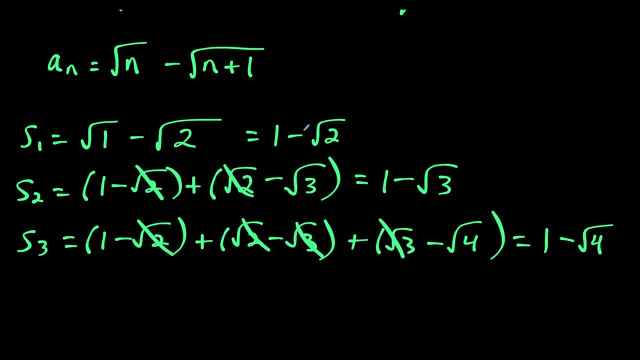 I know this is going to give us 1 minus 2, which is negative 1, but the point is to notice the pattern here. So if we note the same idea as before, that it's always going to be 1 minus square root, and now I look for the trailing square root, the term inside the square root. 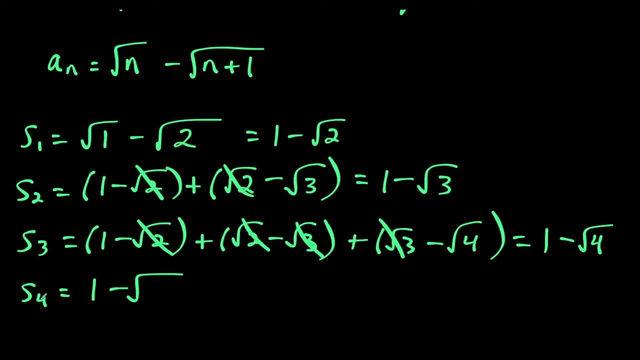 is 1 more than the subscript. So that would tell me this one is going to be 1 more than 4.. This one's going to be 1 minus root 5.. And then from here we could use this to find the nth partial sum. We'll have 1 minus the square root of, and, once again, the 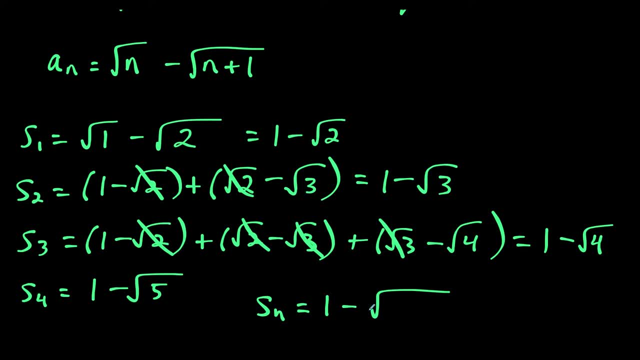 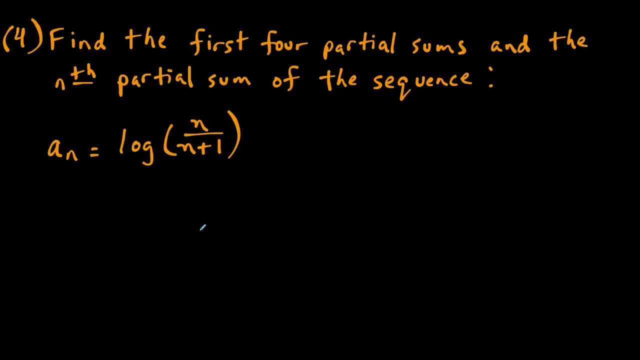 term. inside the radical, the radicand is 1 more than the subscript, So this would be 1 minus square root, n plus 1. So that's our nth partial sum. So for the last example here we have this log expression. So what I want to do is list the first few terms of the sequence. 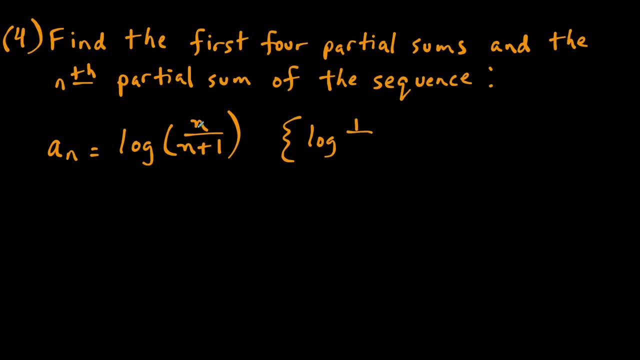 So I have log of. if I plug in n equals 1, I'm going to have log of 1 over 1 plus 1, which gives us log of a half. Plug in n equals 2, that's going to give us log of two thirds, and then we'll have log. 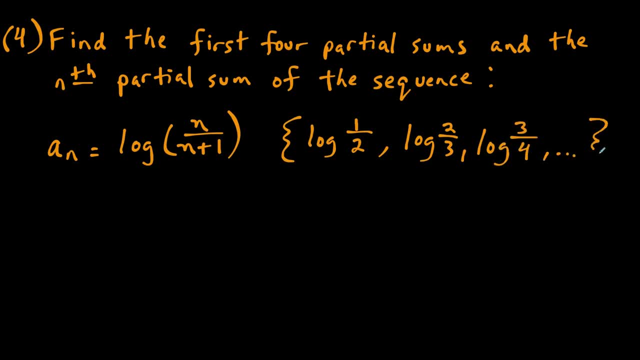 of 3 over 4.. So what I notice here is that when we actually do the partial sums, there's a few ways we could do this, but if we write log of 1 over 2 and then for the second partial sum we have log of 1 over 2 plus log of 2 over 3, we could combine these two logs into a single log by. 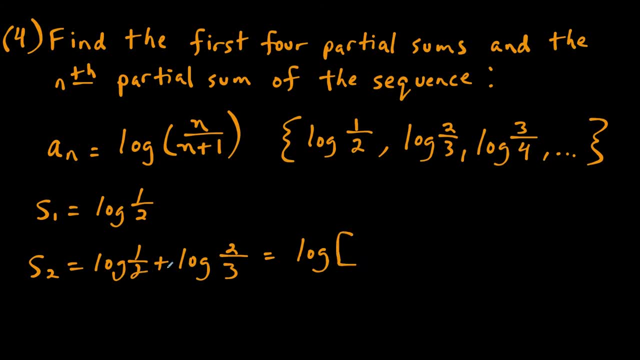 multiplying their inside terms because they have the same base. These are both log base 10.. So this would be log of 1 half times 2 thirds. And notice that 2 over 2 cancel is giving us just log of 1 over 3.. So now, if we do, 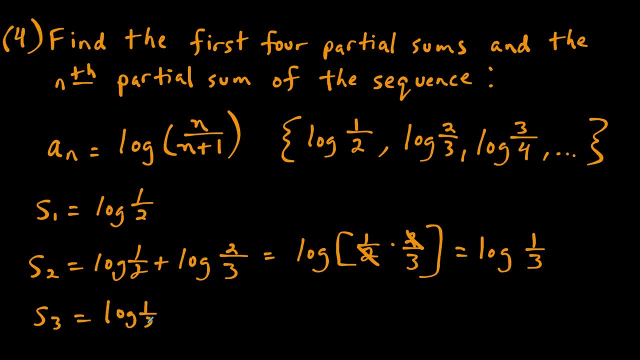 the third partial sum. this gives us log of 1 half plus log of 2 thirds, plus log of the third term is log 3 fourths. So then, same idea as before, that we could combine these logs into a single log by multiplying, But then we could combine that log into a single log with this one by multiplying. 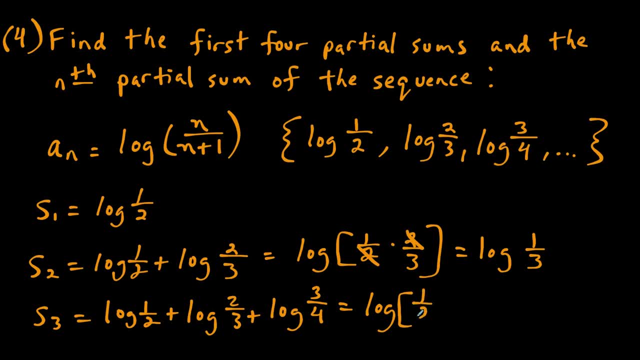 as well. So really what we're doing is we're just going to wind up doing log of 1, half times 2, thirds times 3 over 4.. And if you notice here 2 over 2 still cancels, but now 3 over 3 cancels. 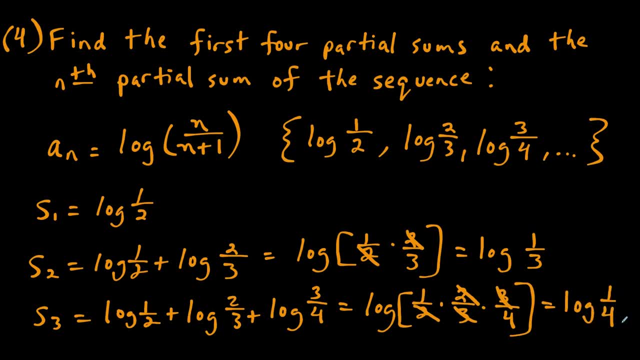 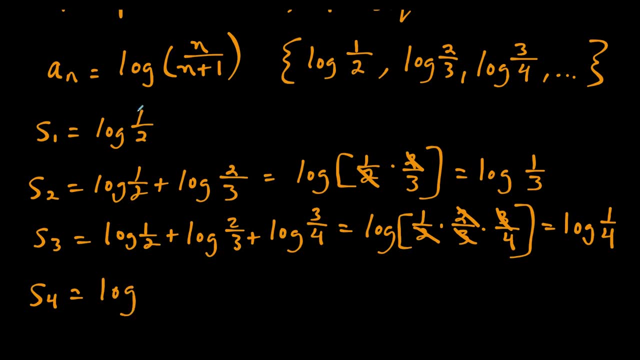 leaving us with just log of 1 over 4.. So the pattern might be obvious If we pay attention to this. here we have log of notice: when it was subscript 1, we had 1 over 2.. Subscript 2, we had 1 over 3.. When we had a 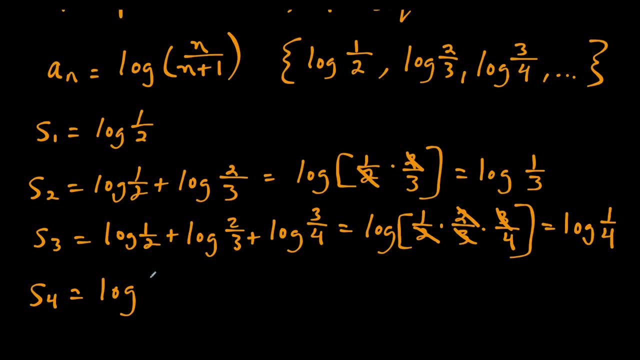 subscript of 3, we have 1 over 4.. So this one's going to give us log of 1 over 5.. So the pattern in general for the nth term is we're going to have log of 1 over, and notice the denominator. 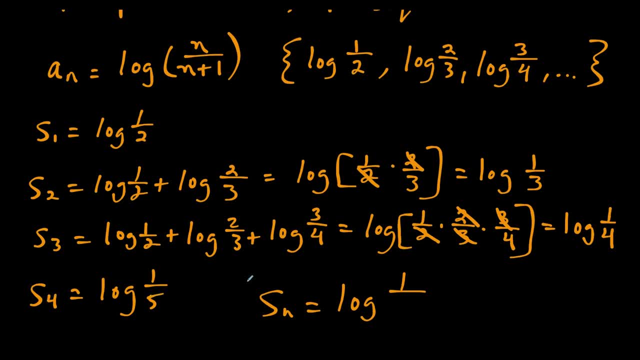 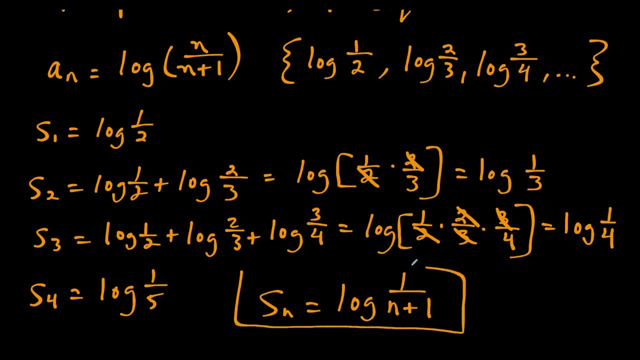 log of 1 over 3.. So this would be log of 1 over 3.. So this would be log of 1 over n plus 1.. So this is our nth partial sum. Okay, well, this is going to conclude this video on partial sums. If this: